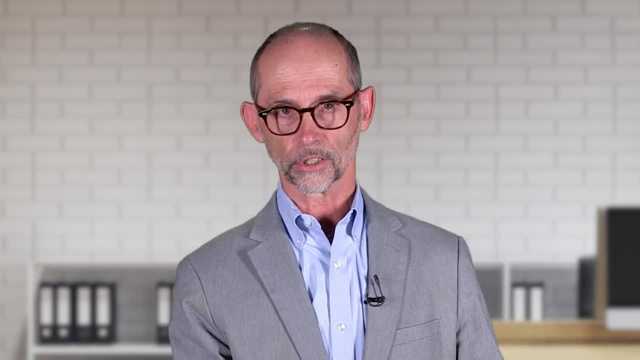 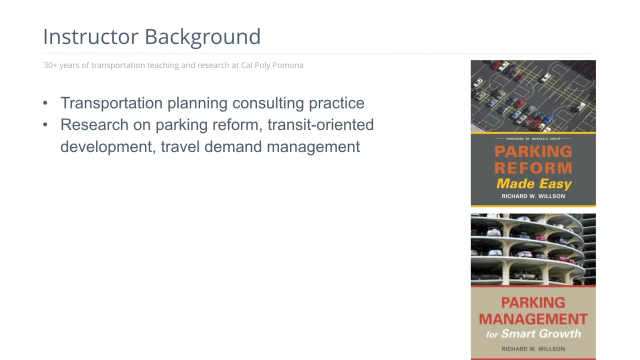 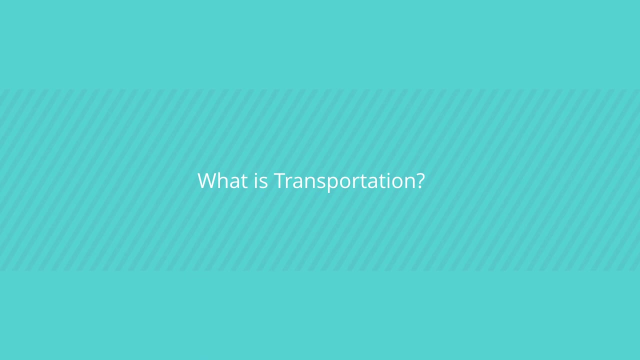 Urban and Regional Planning at Cal Poly Pomona. I've been teaching transportation for my career at Cal Poly Pomona. I also do consulting in parking and transit-oriented development and I've written a couple books about parking reform. I'd like to start the course by reviewing the basic role of 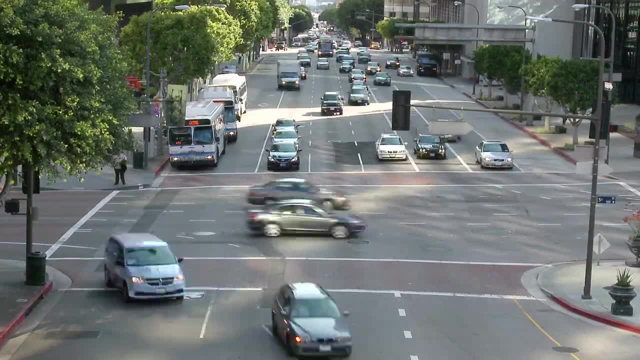 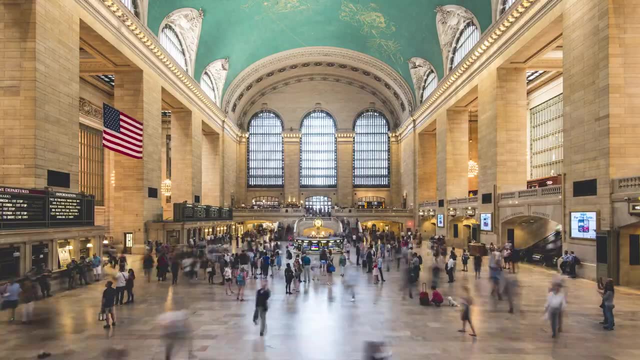 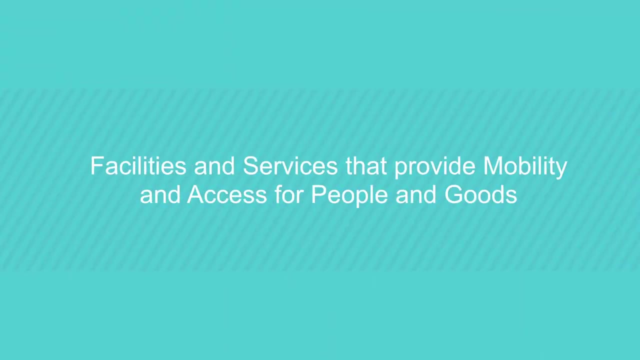 transportation, which enables social interaction and economic transactions: Social interaction being visits to friends. economic transactions being going to work, goods movement and trade. So my definition of transportation is that it's both facilities- roads and rail systems- and services, taxi service, transit. 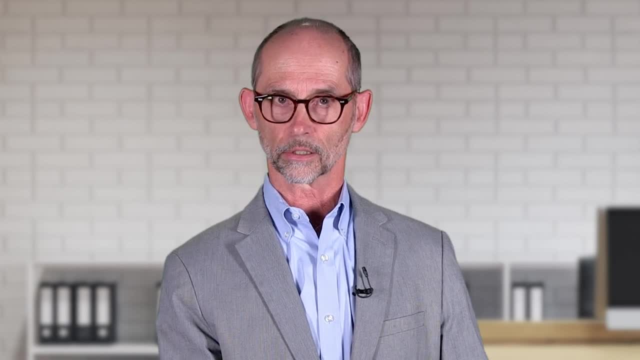 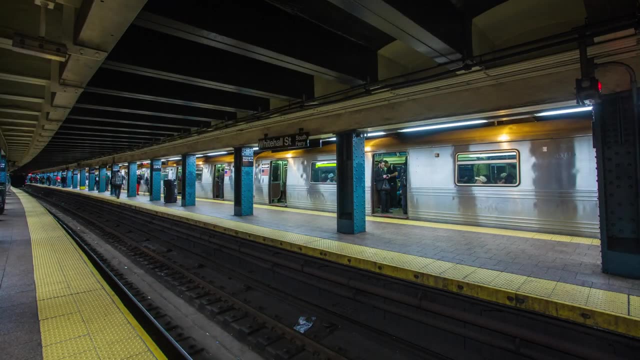 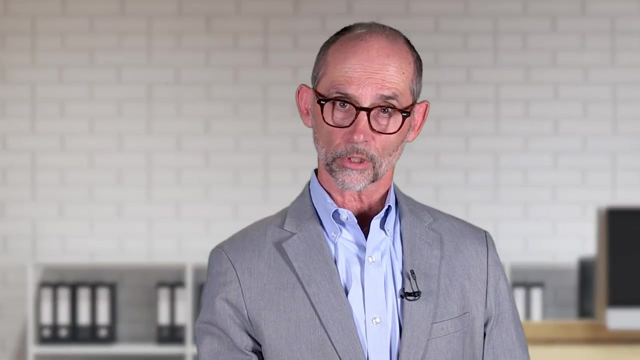 service that provide two things: mobility and access. Mobility is getting from here to there generally, and access is getting from the transportation system to your particular destination, such as from a rail transit stop to an office building or a home. And also it's important to note that the transportation 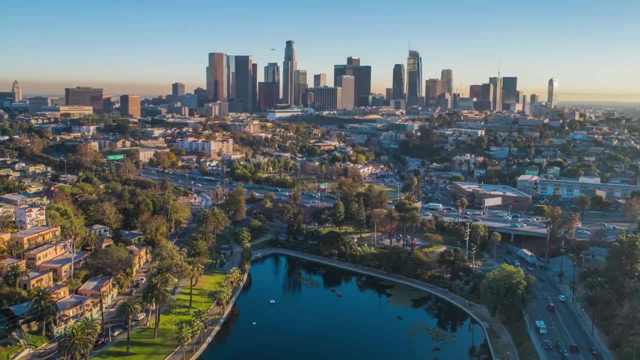 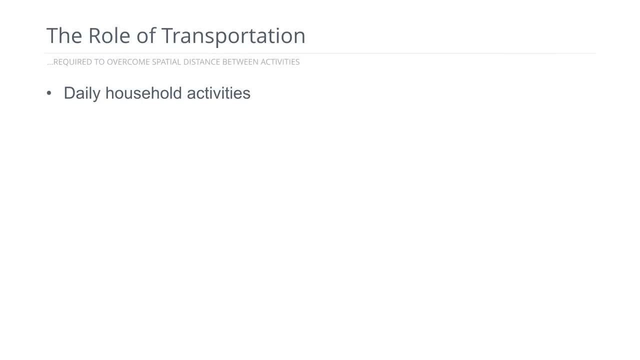 system serves both people and goods movement. So we have transportation systems because we have to overcome spatial distance between activities. So transportation systems serve daily household activities. They allow people and businesses to decide where to locate spatially. They provide mobility for labor, both getting to work and relocating. They provide for economic 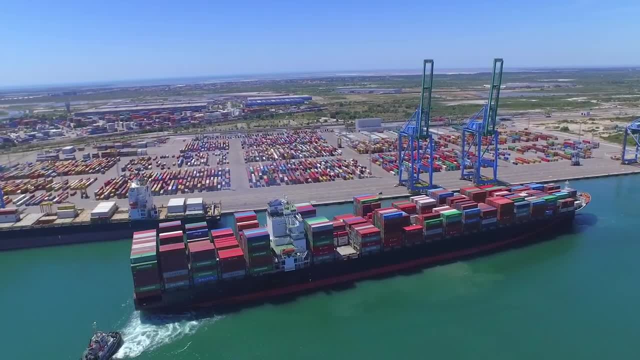 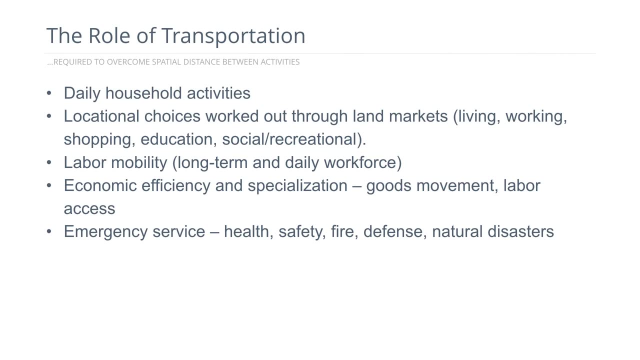 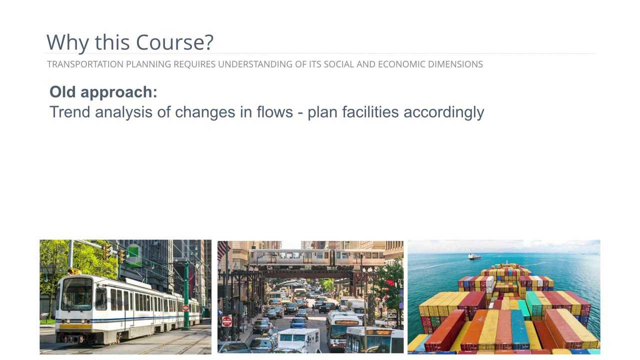 efficiency by allowing regions to specialize in the economic activities they do best. And finally, of course, they provide access for emergency service. So why this course? The key idea is that transportation requires an understanding of social and economic dimensions. The old approach in transportation planning was a trend. 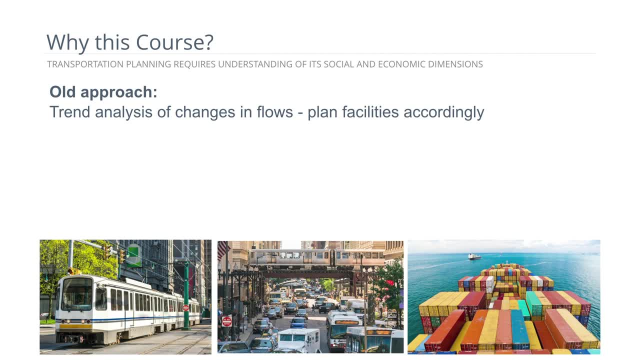 analysis. Is this a busy road? There's a lot of traffic, then we should add to the road or build a new one. The new approach is trying to understand the full dimensions of travel, including why people travel, why they pick locations, why. 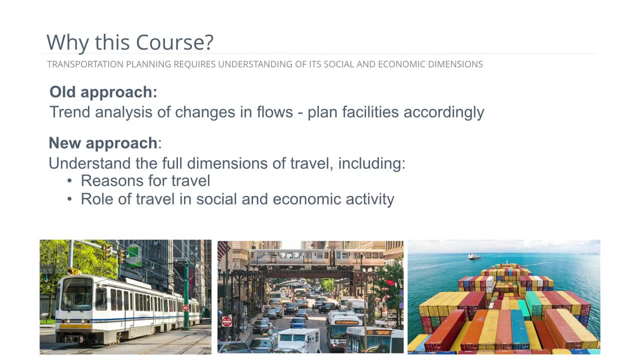 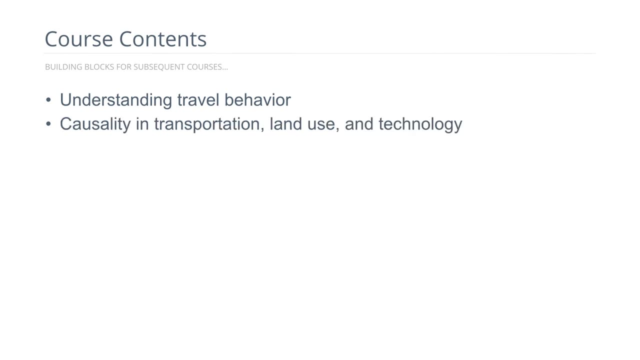 they select certain modes. Understanding the role of travel in social and economic activity and, importantly, understanding likely responses to policy interventions. The course contents include understanding travel behavior, issues of causality and transportation, land use and technology. key transportation concepts. the. 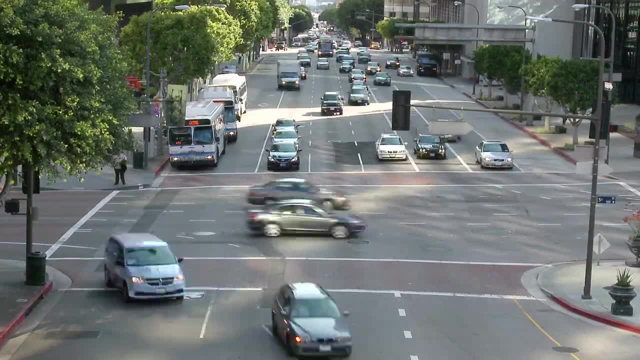 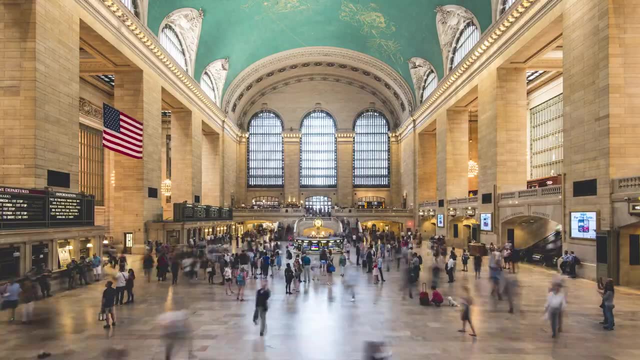 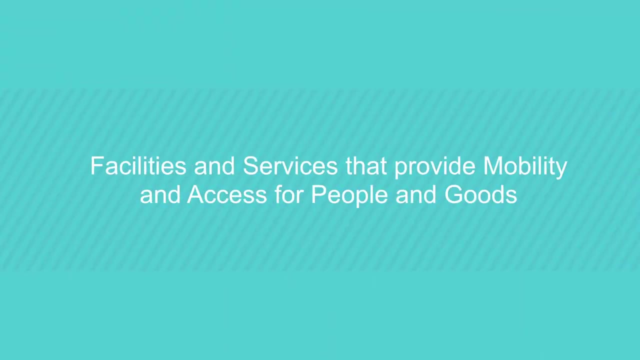 transportation, which enables social interaction and economic transactions: Social interaction being visits to friends. economic transactions being going to work, goods movement and trade. So my definition of transportation is that it's both facilities- roads and rail systems- and services, taxi service, transit. 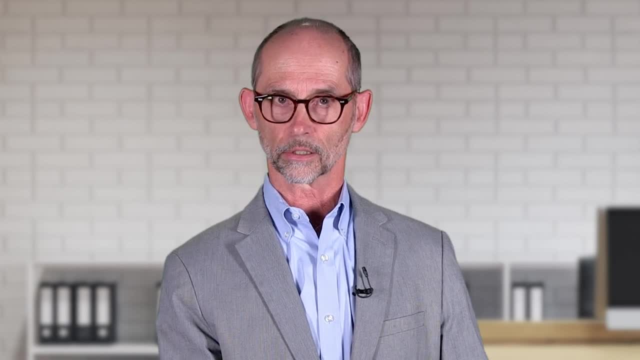 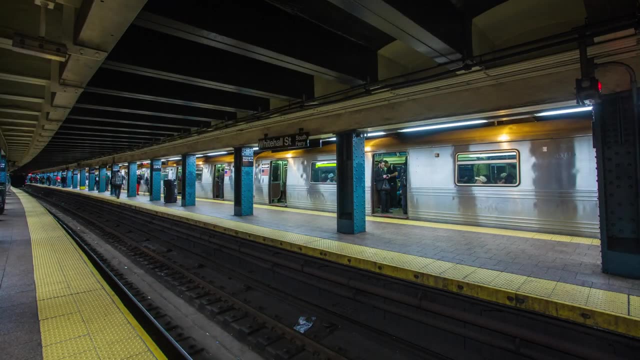 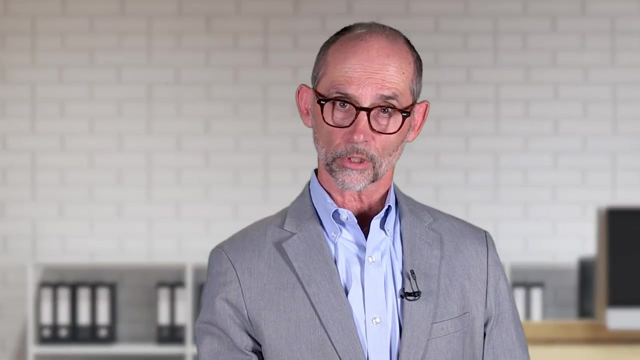 service that provide two things: mobility and access. Mobility is getting from here to there generally, and access is getting from the transportation system to your particular destination, such as from a rail transit stop to an office building or a home. And also it's important to note that the transportation 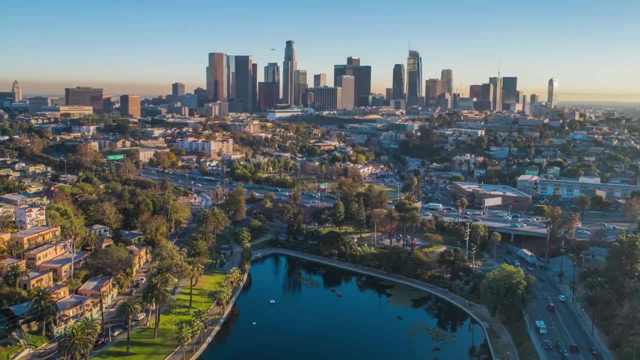 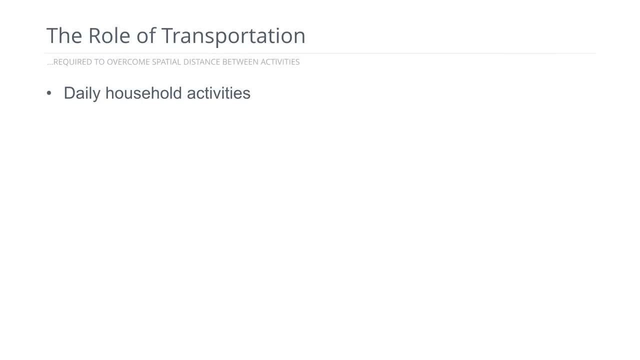 system serves both people and goods movement. So we have transportation systems because we have to overcome spatial distance between activities. So transportation systems serve daily household activities. They allow people and businesses to decide where to locate spatially. They provide mobility for labor, both getting to work and relocating. They provide for economic 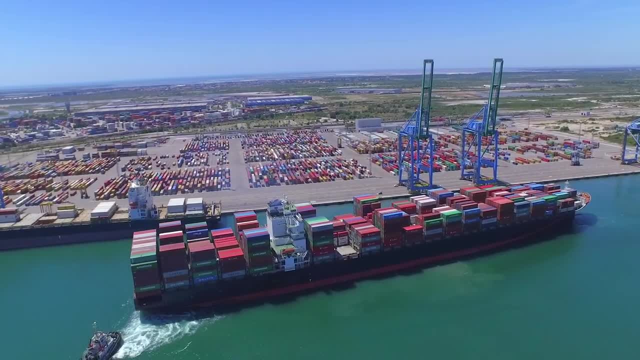 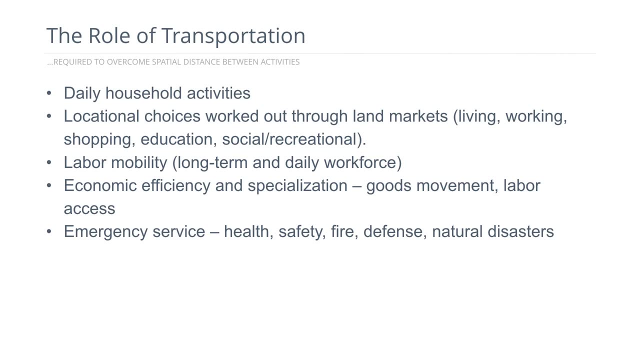 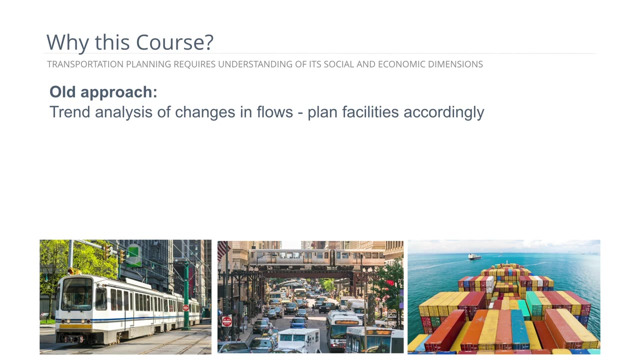 efficiency by allowing regions to specialize in the economic activities they do best. Finally, of course, they provide access for emergency service. So why this course? The key idea is that transportation requires an understanding of social and economic dimensions. The old approach in transportation planning was a trend. 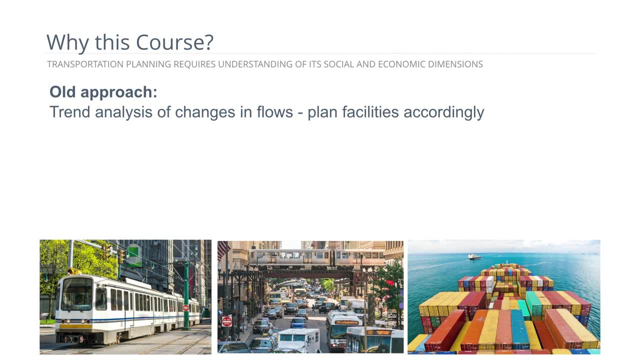 analysis. Is this a busy road? There's a lot of traffic? then we should add to the road or build a new one. The new approach is trying to understand the full dimensions of travel, including why people travel, why they pick locations. 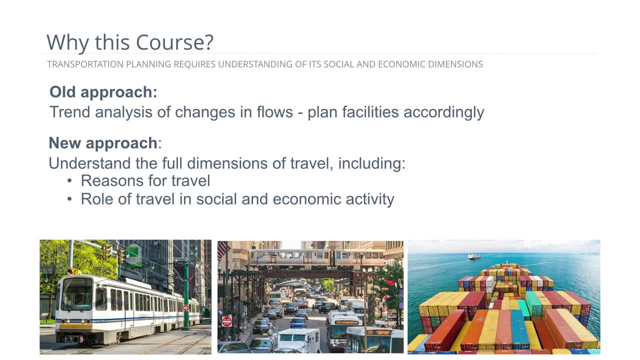 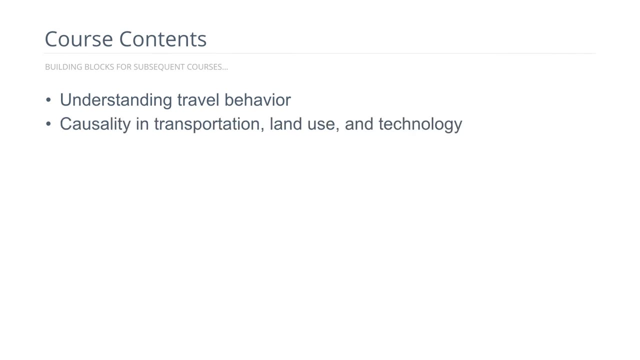 why they select certain modes, Understanding the role of travel in social and economic activity and, importantly, understanding likely responses to policy interventions. The course contents include understanding travel behavior, issues of causality and transportation, land use and technology, key transportation concepts. the. 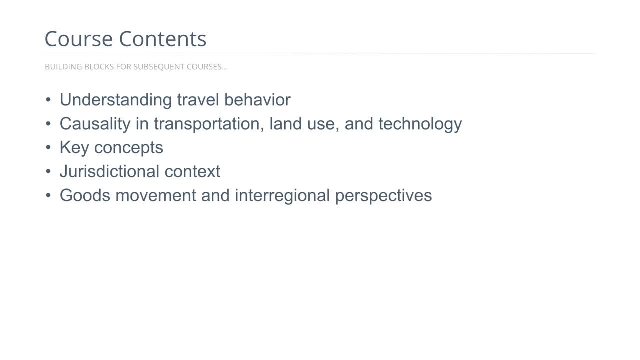 jurisdictional context for transportation, goods movement and inter-regional perspectives. And finally, we'll conclude with a discussion of the future as evolution or revolution. Now let's get started.